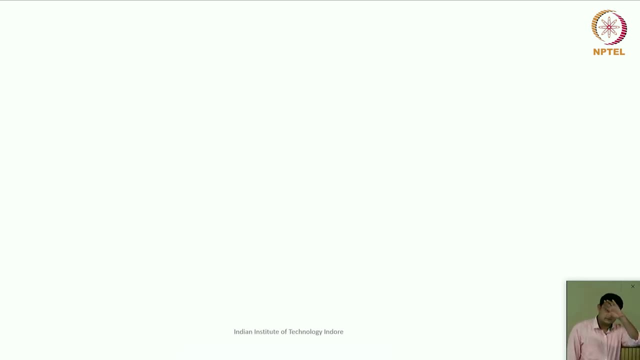 the communication is basically: you see a padlock at the top and it is written as HTTPS. So here HTTPS means HTTP is an application layer protocol. that S stands for security. basically it is operating over the SSL communication. So that is the roughly the idea. 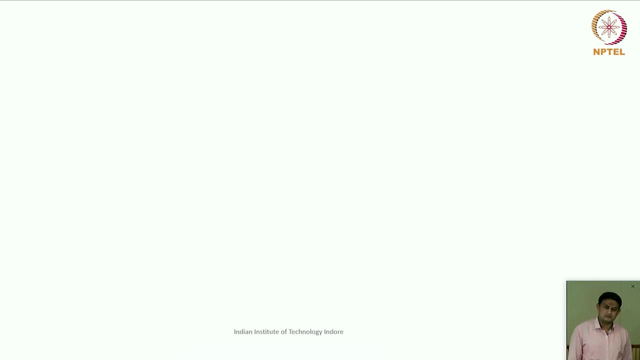 So what we want to do is how exactly this security is given to the HTTP inside when it communicates. So that is what the goal. So, just to recap your memory and give some context to the discussion, what we saw in the previous lecture is: 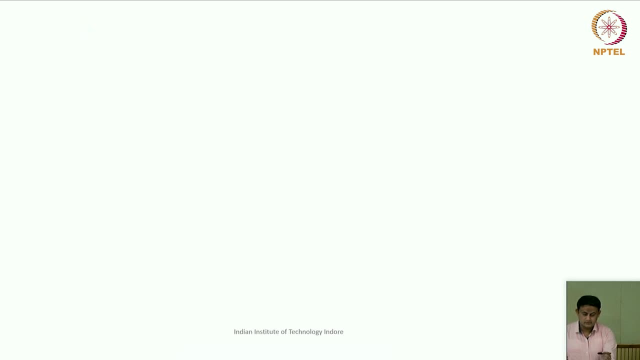 So if you look at, we saw the email. Email is one application whenever email is sent. So this is- you can think of this as application layer, and then below that you have the transport layer and below that you have the network layer, and below that you have the network layer. 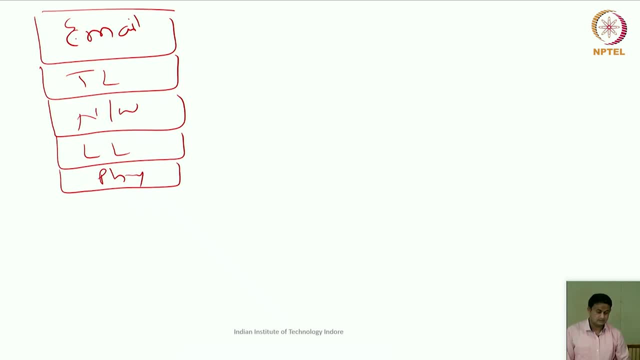 So this is the link layer and then the physical layer and on the other side also, you got the similar structure: the physical layer, the link layer, the network layer and the transport layer and finally the application, which in this case is the email application. 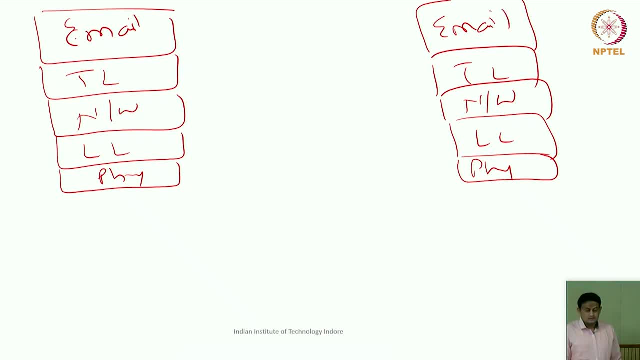 So when we send the data from the email, So when we send the data from the email, So when we send the data, So when we send the data So from, particularly when I send an email from my system, So when it is supposed to go to the other end, when somebody who is the Internet Receipt. 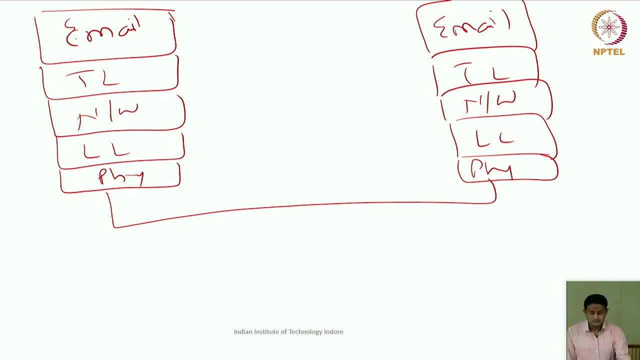 receives that, so that is also an application. So when we discuss yesmime, Yesmime operates at this layer. So whenever something is encrypted, it is encrypted at the application layer. So email content is encrypted, encrypted and the S-MIME itself is operating or working. the implementation of the S-MIME. 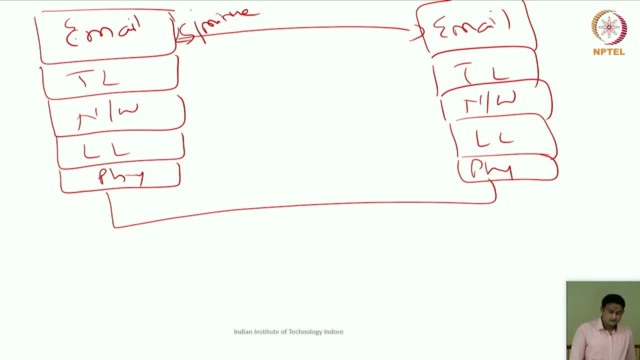 itself is at the application layer. so this is the. compared to that, the difference between the TML communication and the TLS or the SSL is, unlike the previous S-MIME, this operates at the more or less at the transport layer. here we are talking about the. it is not exactly. 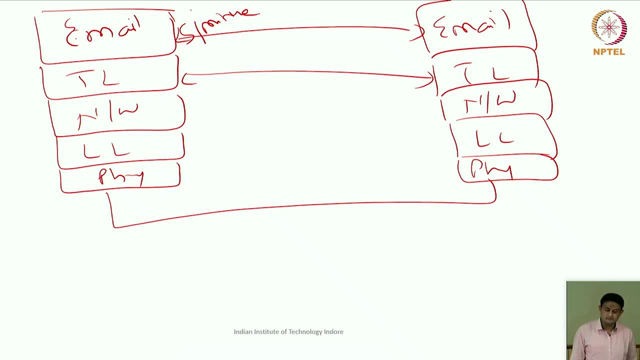 at the transport layer you can think of in between the application layer and the transport layer. so the advantage that goes with the SSL or TSL, by operating at the transport layer or in between the application, the transport layer, is you can use the TLS or the SSL for 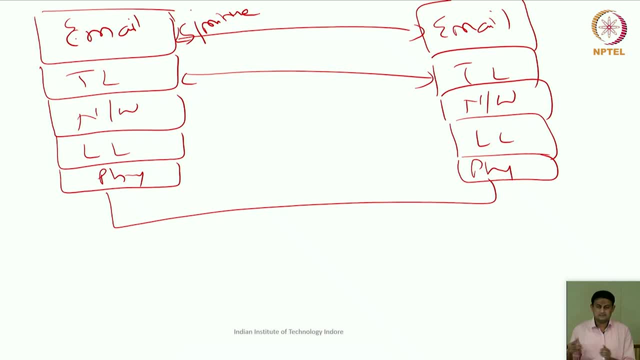 many applications. That is fine. What you cannot do with the S-MIME. S-MIME is only meant for encrypting or providing the security to email communication, and nothing more than that. you cannot use it for HTTP or other similar applications, So that is one difference. 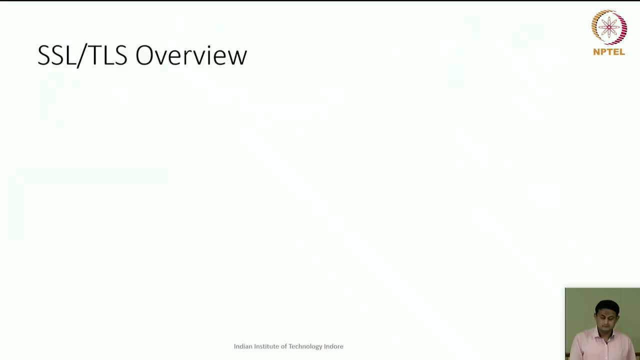 So, with that background in mind, let us see what is the SSL overview is. So. it is meant for providing reliable end-to-end communication. Two parties are engaging in some convergation and what SSL says is: for the applications, you give me the data, I take that data and then I transfer it to the other end by providing. 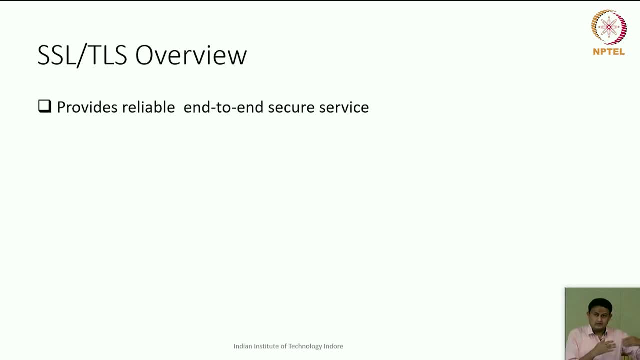 the security, which is the encryption, and the application at the other end can actually pick up the data from that tunnel and then process the data. so that way the security is end-to-end And then the other end can actually pick up the data from that tunnel and then process. 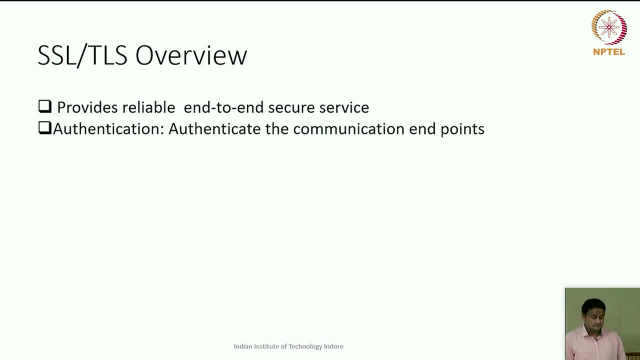 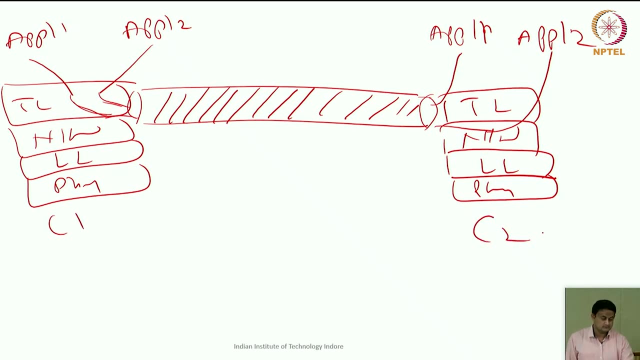 the data, so that way the security is end-to-end. And then, in addition to encrypting the data that is transferred with the two ends, it also authenticate the peers who are engaging in the communication. If you go back to the slides, what it says is: this is client 1 and this is client 2, or 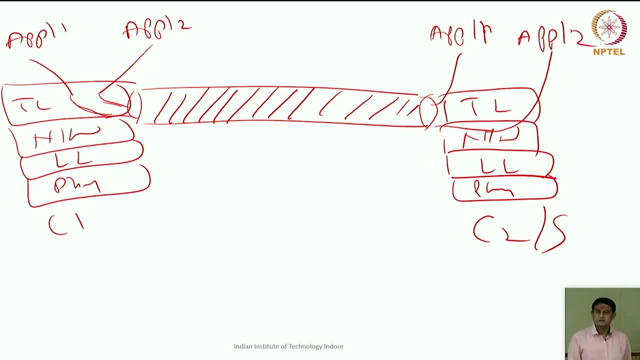 you can call it maybe, as a server doesn't matter. So the client is authenticated to the server and the server is authenticated to the client both ways, Although practically, at the end of the day, it is not a server, it is a client. So when you deploy it at the implementation level, when you deploy it, particularly if you 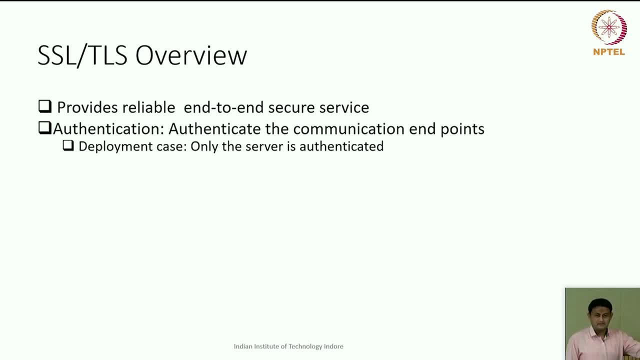 take the case of the STTT: typically what happens is only the server identifies itself. So when I do the transaction with in my bank account, I am my client or I want to make sure that I am indeed exchanging the communication or establish the communication with the banking. 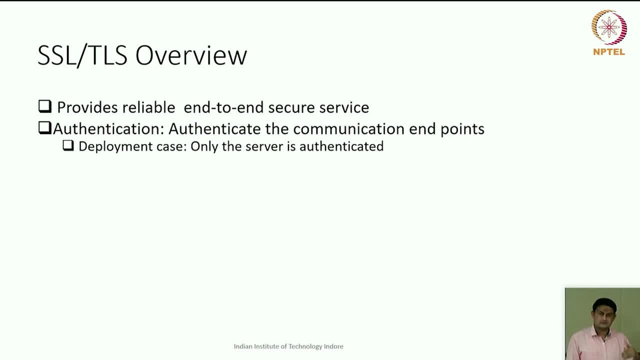 server, nothing else. The server identifies itself, meaning the server is authenticated, And in most of the cases, the client is not authenticated to the server. It doesn't matter who the client is. who is actually engaging from where I log in. So, whether it is the system number 1,, 2 or 3, as long as I provide the right credentials. 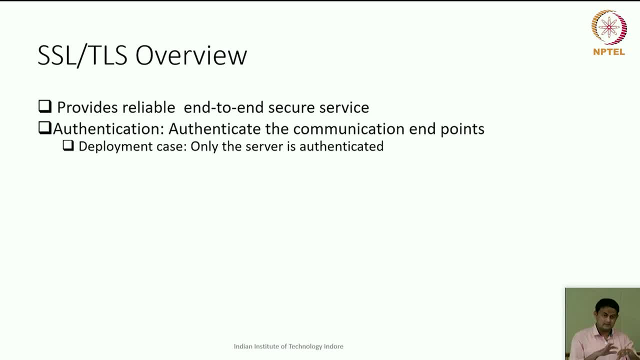 to the application layer. when I give the my username and password at the my bank account, it's actually the authentication is at the application layer. When I am talking, the authentication now with respect to SSL, It is the transfer layer authentication. So, although you can use authentication mechanism in both directions, but most of the times in 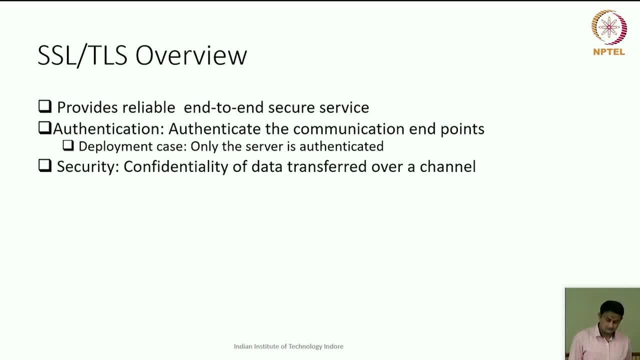 practical use cases, it is only the server which actually authenticate itself And, as we discussed, it provides the competency if the data transferred. how do it does? by encrypting the data that is transferred. So, but one difference is encrypting the data, But one difference is encrypting the data. 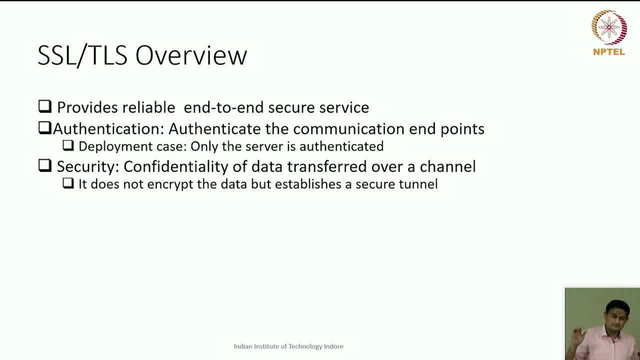 But one difference is encrypting the data. It means that when I am operating at the application layer, I take pieces of the application, whatever chunks that is given, and then I encrypt those messages. But here what the TLS or the SSL says is: you give me any byte stream, as long as it is I. 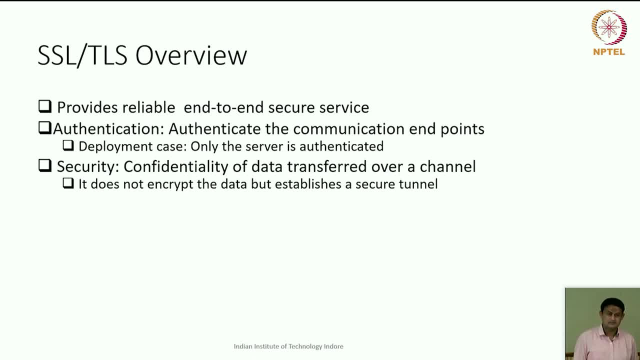 receive something from the application. I am just encrypting that, So it is not encrypting the message per say every message. So message 1, message 2, message 3, there is no difference like that. I just take the raw data as it is and then encrypt that data and transfer it to the other end. 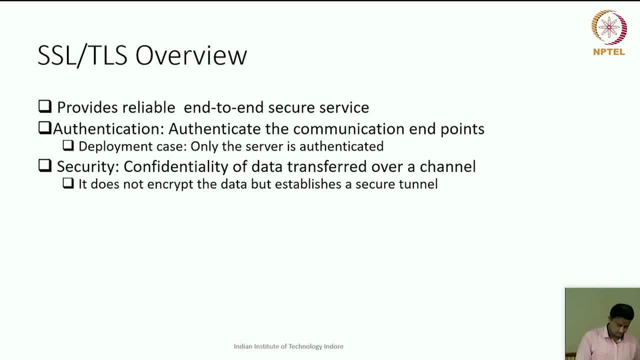 That is the meaning of the SAP security secure tunnel And, as I said, it is application agnostic. It is meant to be used with respect to different applications. So, if you use the SSL or the TLS, what it provides is it prevents eavesdropping. 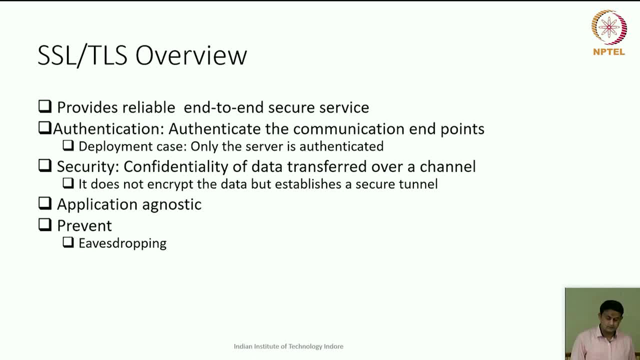 Somebody who is sitting in the middle of the conversation cannot actually make out what is going on because everything is encrypted. It also provides security against tampering, So somebody who is sitting in the middle cannot actually manipulate the data that is transferred between two systems. 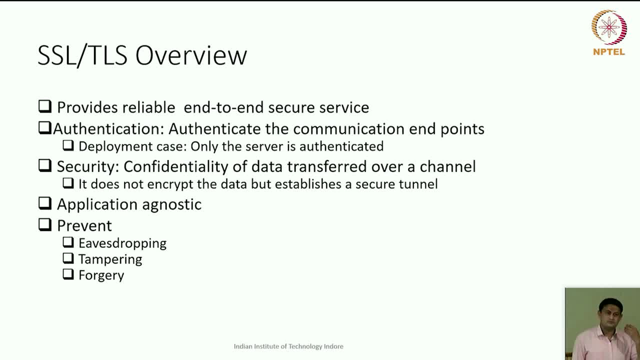 And somebody cannot fabricate a message. it cannot. origin claiming to be other party sending the data is actually one new message cannot be fabricated and sent to the other parties, So it provides all of this. that is essentially what we discussed in the first lecture. we required that confidentiality, integrity and the authenticity of the data. 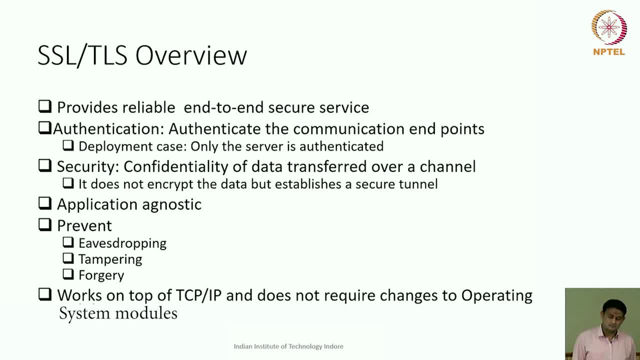 So, in nutshell, SSL or TLS provides all of them. So, although we didn't talk about integrity as of now, but it is also there And its biggest advantage is it works on top of the TCP And, as a model you can insert, it does not require any changes to the operating system. 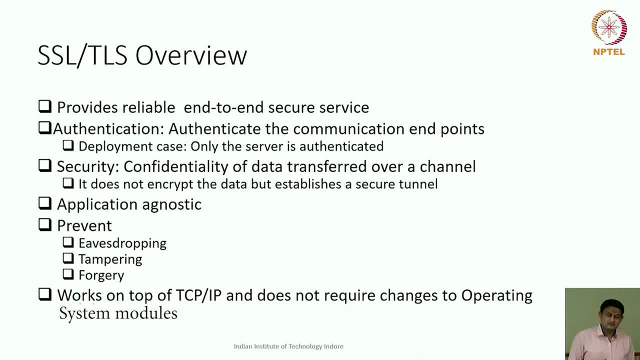 kernel. Typically the TCP IP stack that we use is implemented as part of the kernel in the operating system. So if you have to change that, then it's actually a little tedious. But a good news is SSL doesn't require any of those changes. 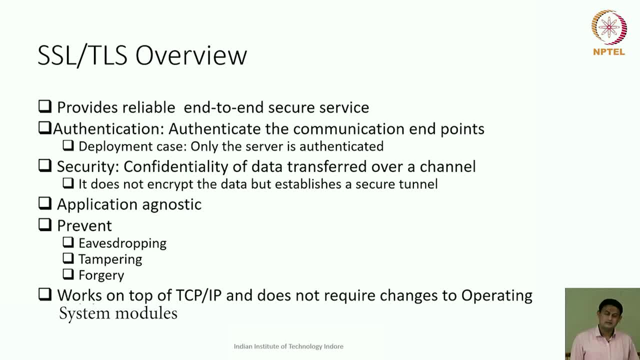 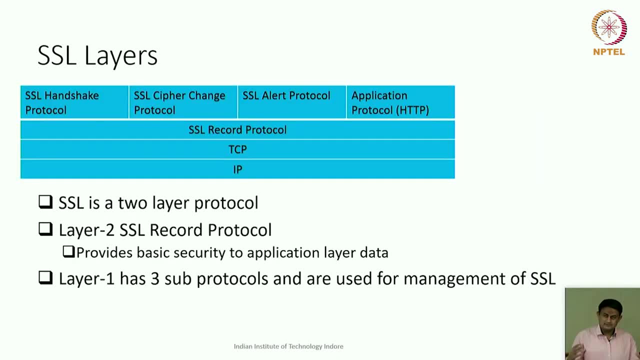 So it can directly go and sit on top of the TCP IP stack. Okay, It is not a simple protocol that starts functioning. So SSL is not a single protocol which does all of this. It has four protocols. One is the major chunk, which actually does the work, is the something called SSL record. 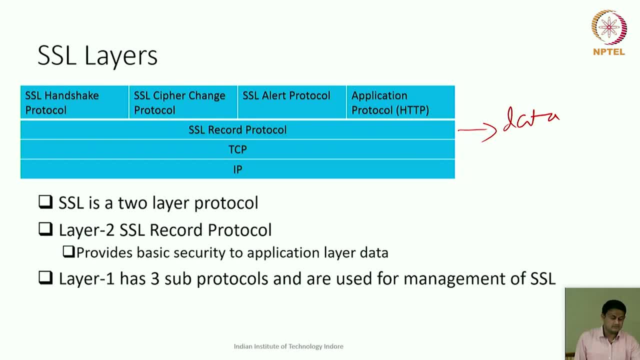 protocol. This is the one which encrypts the data and also provides integrity of the data. whenever I use this protocol, I use this protocol and transmit it, and that you can call it as layer one or two, generally called as layer two. so this is layer one layer of the SSL protocol and that sits on top of the TCP. 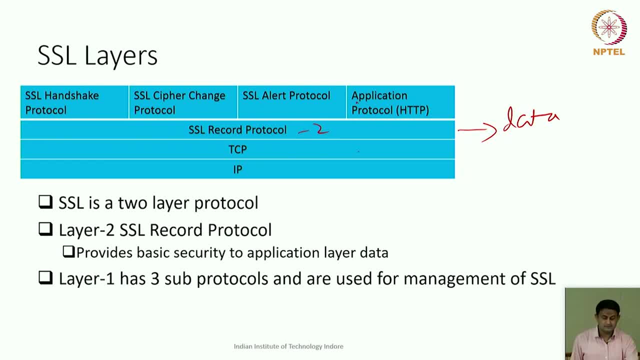 so application is here, TCP is here in between these two. this protocol actually functions in between the TCP and the HTTP or any other application. and on top of this above layer or layer one, it has got three sublay protocols. so one is called SSL handset protocols, the second 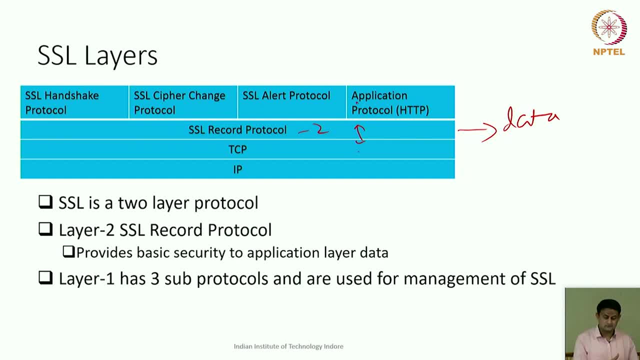 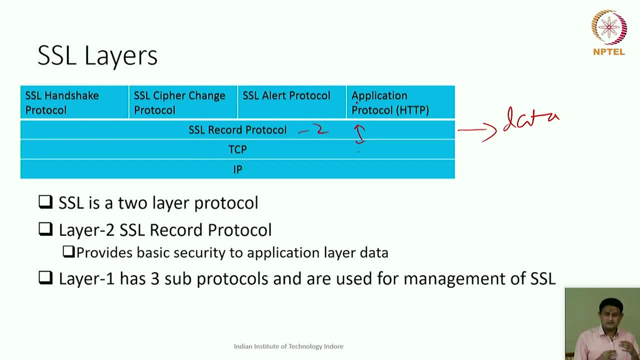 connection between the two end systems and then a kind of monitor what's going on between these two, whether things are okay or something need to be changed, or is the other party need to be alerted or stuff like that. so in actual, this is what the management, operation or the control. 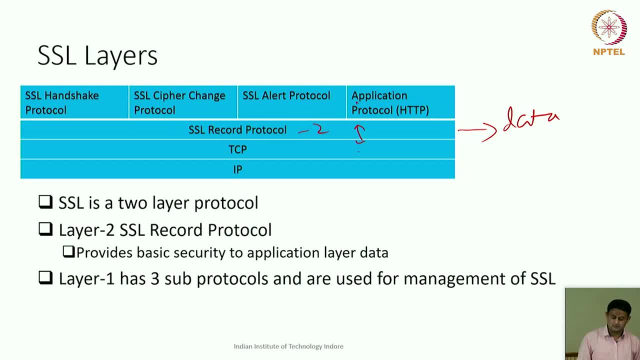 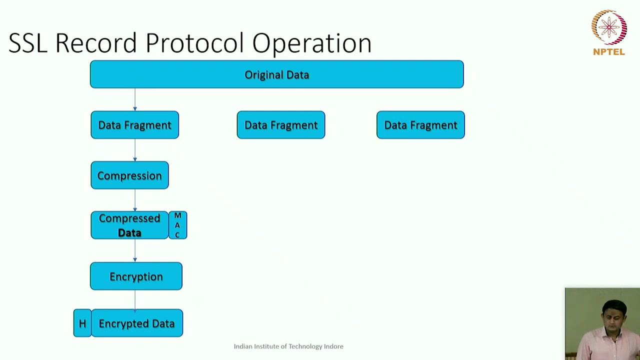 plane operations are done by these three protocols, which are at the layer number one, and the actual data transfer, the encryption, whatever the application is giving, that is carried over the SSL record protocol. so let's take a look at how, what are the details of these protocols, in fact each one of them, and then see what exactly happens there. so, to begin with, 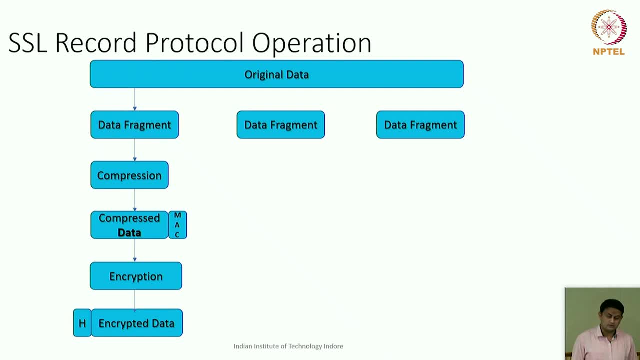 let's start the discussion on the SSL record protocol. so this is actually the heart of the SSL. whatever the encryption or the whatever data that is transferred, it is actually transferred through this. so what it does is it receives the raw bytes from the application, so the original data that return is: this is the application. 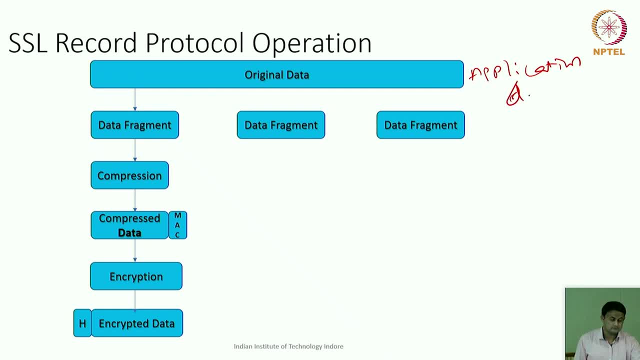 data so that application data- this might be the data given by HTTP- take that data and then divide that data into fragments- so small chunks, so raw bytes. you take it and then you divide them, bunch them into fragments. so the SSL puts a limit on the quantum of the data that can go inside. 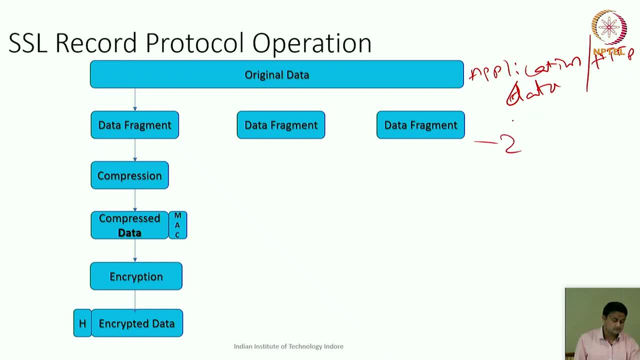 one fragment that turns out to be at the max 2 to the power of 14 bytes. so in one chunk or in one fragment you can have these many number of the bytes. this is the maximum limit, so you cannot carry beyond that. so it can be actual data can be smaller than this. 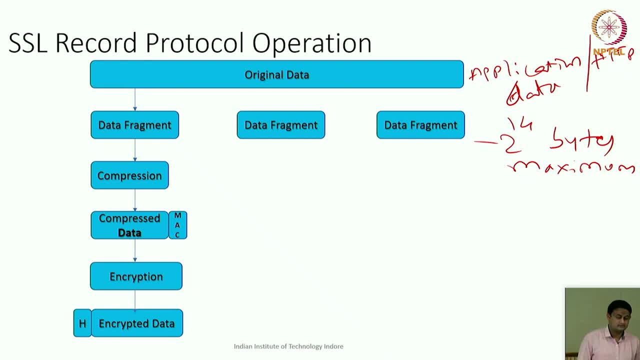 but there is something that is done, so we will come to that in a minute. So at the max 2 to the power of 16 bytes, and the data can be less than that. so once you fragment that data, the next step that happens is you use a compression algorithm and then 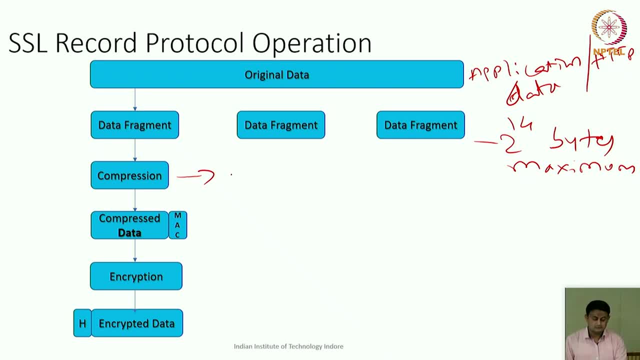 try to compress that data. So this is actually a lossless data. Lossless compression meaning data is not lost. there are, whenever you talk about the compression algorithms, there are two types. one is the lossless, second one is the lossy. 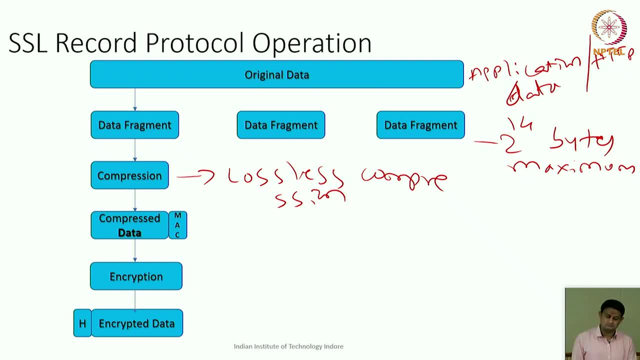 compression. Lossy compressions are not used in typically HTTP communications, but sometime in other domains. maybe if you want to compress an image or a video so that time you can afford to lose some information in the image, You can make the image. 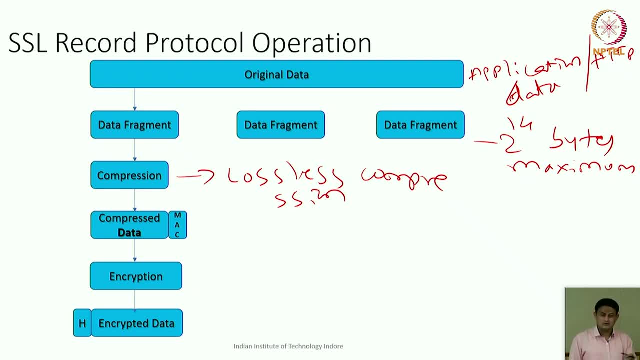 If the image is slightly blurred and lose it, that's okay, But not here, in this context, when you use the for banking transactions, we don't want. if you transfer a million dollars, the leading one is actually disappeared during the compression. 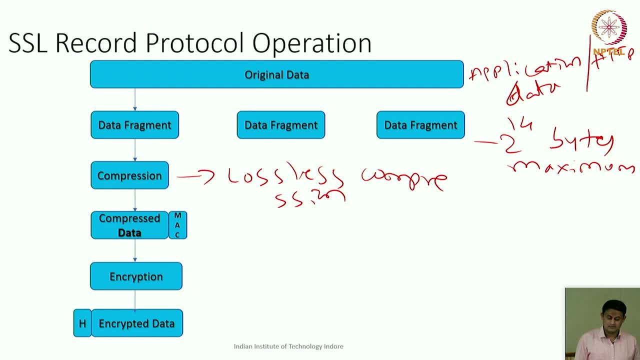 that should not happen, So it actually doesn't allow that to happen. So compression always does not necessarily need to reduce the size of the data, but sometimes it can, also because it's not lossy. so it might if you transform the input data using 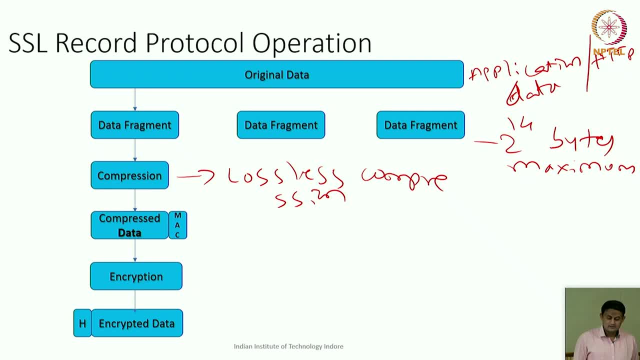 an algorithm, it might slightly increase as well. So, then, SSL actually puts a limit on how much that increase can be. The compression can, reduction can be up to any level, but the increase can be limited to certain points. So, once you apply the compression, you take that compressed data and then, at the end of 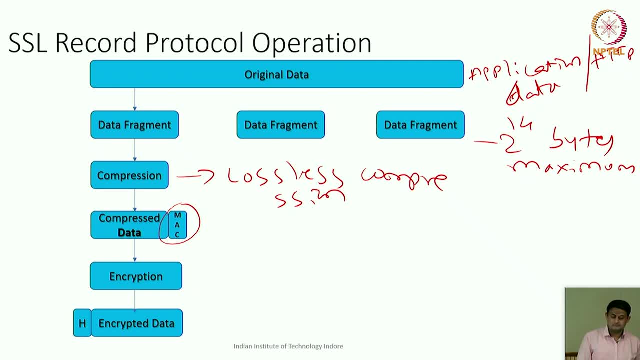 this: you append something called as the message authentication code, or called as the MAC. So MAC is simply the. you take the hash algorithm along with the key and then you attach that. So basically, this is a hash algorithm, but it has got a key. 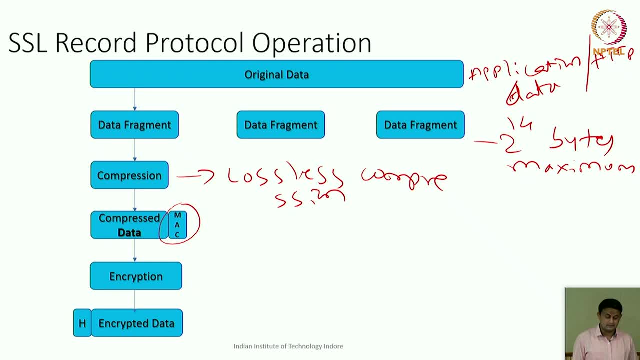 So we did discuss this- how the MAC is generated. In the next slide I have got the details of exactly what this MAC is calculated For the time being, assuming that is there on the, but it is calculated on the compressed data. 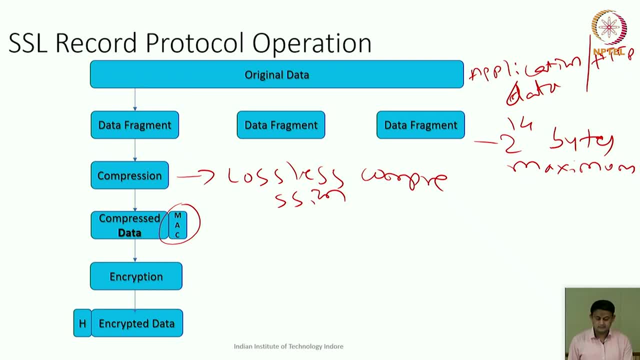 Once the MAC is attached on that, you take this whole bunch- the compressed data and the MAC itself as input, and pass it on to an encryption algorithm. So that'll bring the security to the data that is emitted. So the data becomes random. 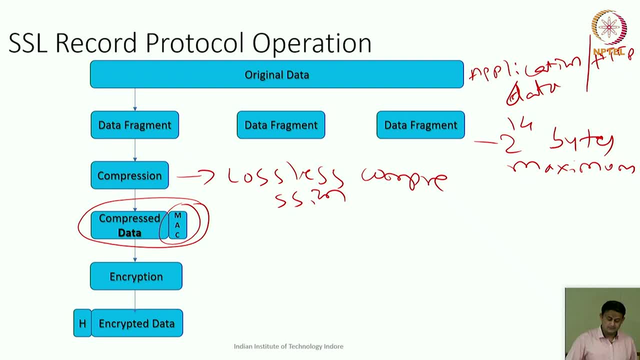 So once you encrypt that data, then after this encryption you attach a header known as the SSL header. So you take the compressed data plus the MAC, encrypt it and then on top of that you attach this SSL header and then transmit it to the other end. 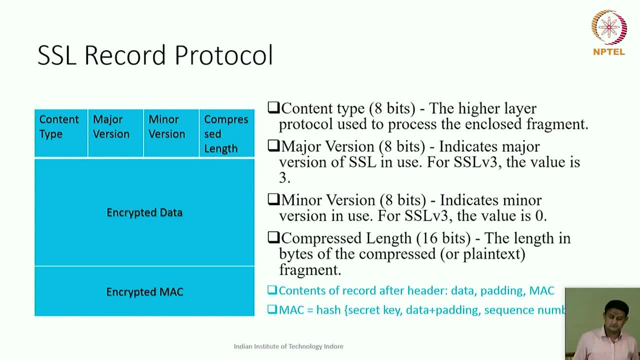 So let's take a look at how the entire bunch look like. So this is the encrypted data, is what the compressed data that I was referring to, and this is what the MAC is. So MAC is one component, the encrypted data is another component, and on top of this, you 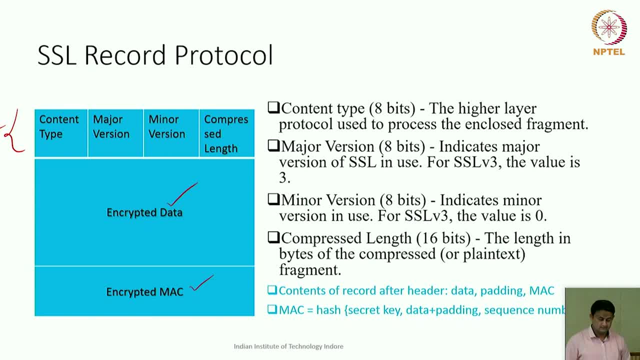 attach this. this is the SSL header. It has got these many. the header has got these many four components. Basically, it identifies what is the application data the SSL protocol is carrying. that is, the content data, The first element within the header, and then it might be HTTP or other applications. 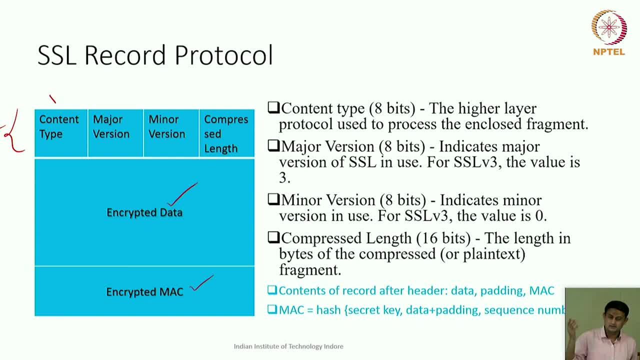 So if you use, for example, FTP, so it tells that this data is actually belongs to an FTP application or HTTP application, something like that. And then the second component is something called as the major version. So this major version is the SSL. 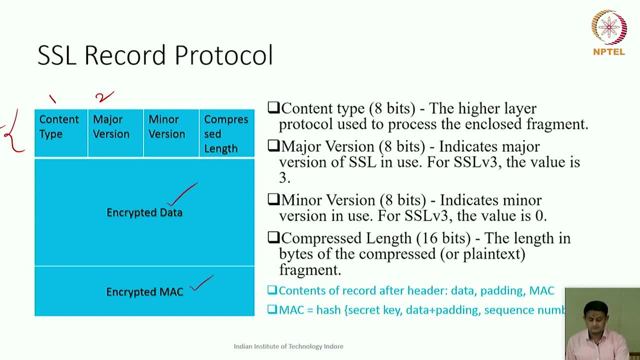 So the SSL stock at version number three. most of the cases it is. if it is in SSL, then it's a version number three And then there is a minor version. sometimes, historically, when it was early stage of the development, people used version number one, 1.1, something like that. 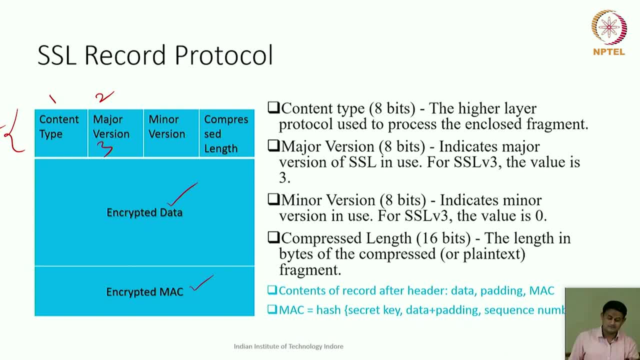 So that is where the SSL stopped, is version number three, and the minor version is usually set to zero And then subsequently the SSL, So the second part, So in some cases the first environmental version and then the second one is the MS. 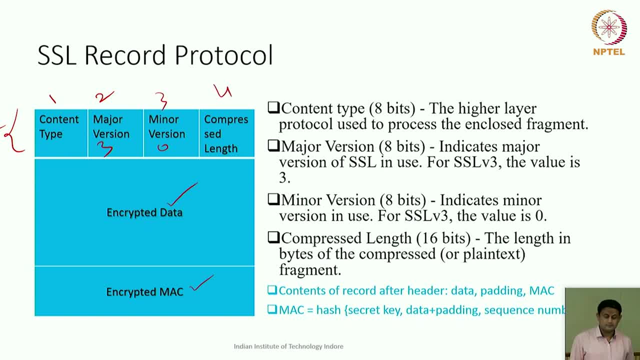 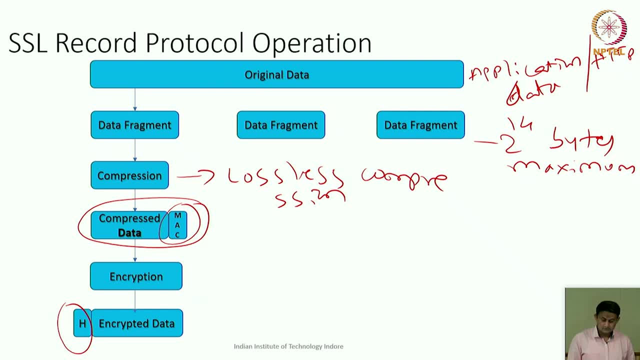 this is the third component, and the fourth component is something called compressed length, So length of the data after the compression, whatever is here, once the compression has happened. what is the length? Let's say here 100 bytes. I am saying the 100 bytes. 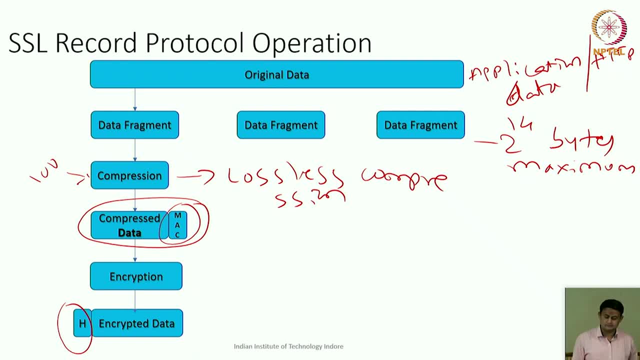 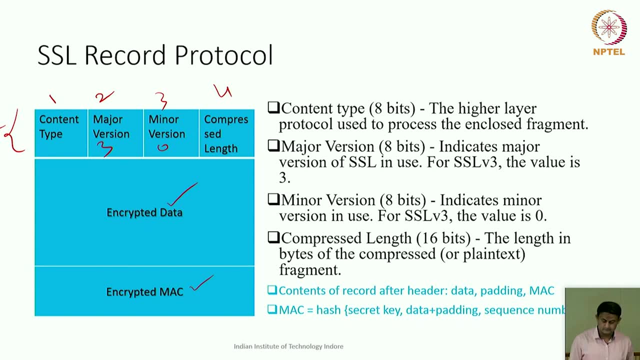 So sometimes to make it work with other algorithms for calculation of the math or the encryption they do require, particularly to use the block ciphers for calculating, encrypting and calculating the hash values, then they do want the data to be of certain length. At that point of time, what can? 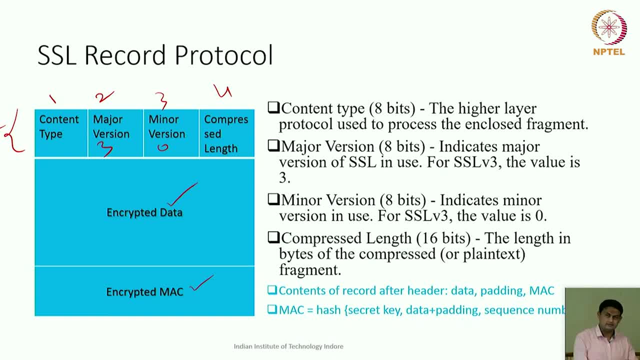 happen is if the data is not exactly ending at the block that the algorithm wants. so at the end you put some kind of padding, So the data all the way from here to here. adding this is the last portion, as you can call it as the padding. 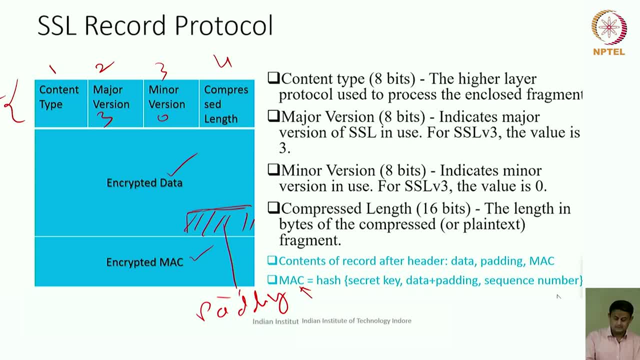 So this padding is data that gets added to just make it multiple of whatever the block cipher requires. so you use this padding and this hash is actually calculated, but the hash, the MAC, is actually calculated using, on top of using this, this padded version of the data. 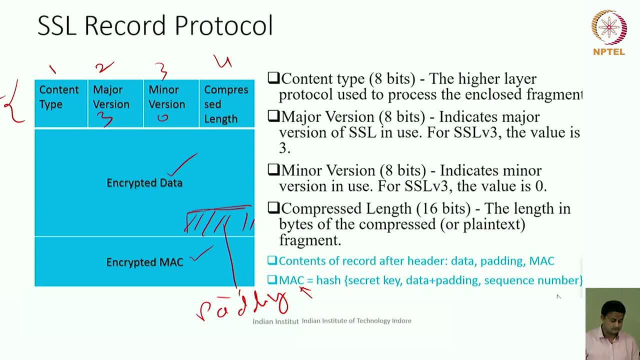 So you take these many components. one is something called as the secret key and the second one is the data and data and plus the padding that I was talking, and then the sequence number. In SSL protocol, every piece of the data is actually identified by sequence number. This is a different. 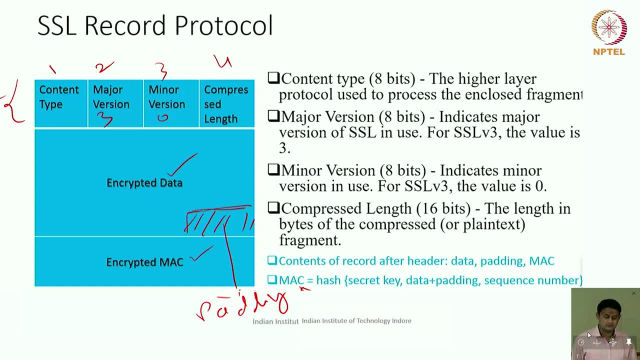 sequence number than the TCP users. TCP also a sequence number, but they have nothing to do with the SSL sequence number. so this is the application data, that the sequence number of the SSL protocol itself, not of the TCP. so that is how the MAC is calculated and that MAC is the one which goes here and then gets. 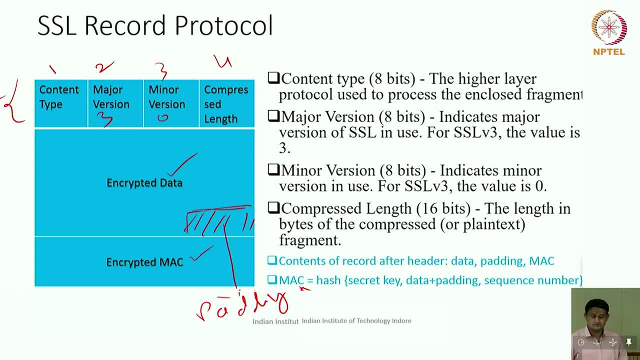 encrypted. so that is what happens in the SL protocol, so that SL particular recorder protocol. so very simple operation. all that you do is take the data, divide that, compress it and then calculate the MAC, including the padding and the sequence number, and attach the MAC to the end of the compressed data. end of the compressed data means plus the padding, plus. 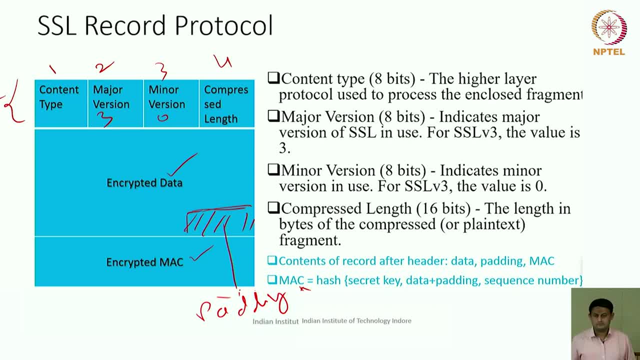 the data and then you encrypt it. after doing the encryption, you attach the header, so it has got these many details, and then you send it. So that is the, So The simple operation of the SL protocol. so this happens in both the directions. so whenever 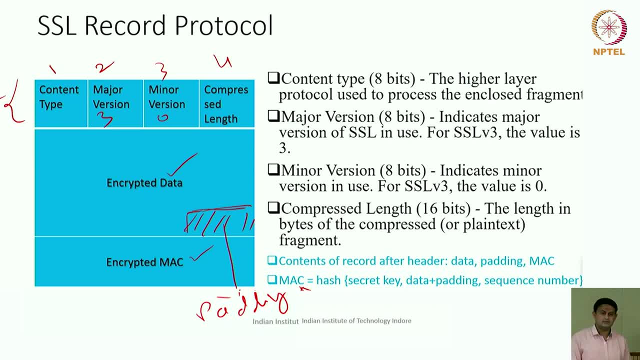 client wants to send something to the server- if you take the HTTP as an example- or the server wants to send something back to the client, in both directions, so this message structure is used. so that is about the SL recorder protocol, the actual data transmission. but now let us take a look at the management protocols that I was referring to earlier. 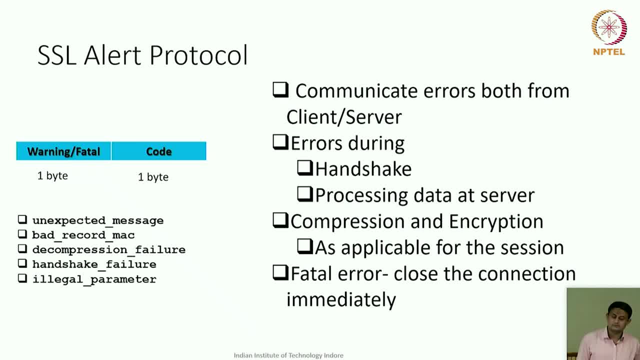 so the first management protocol will begin with the something called as the alert protocol. so alert protocol is mean to communicate the errors and the warnings that are generated during the communication. So those errors might be at the client side or the server side, it might be just any warning. 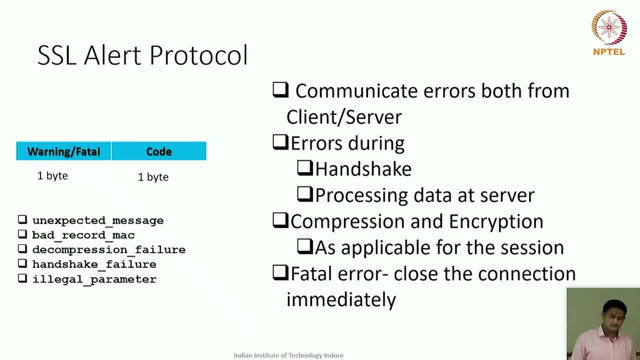 which you can view with, or it can be a message which is you to something called as let us call the alert prot, alarm point or tail point, basically such a message which is used if you are drawing Produkt code. like what else Fidus said earlier: never speak possible words or any of this éto. 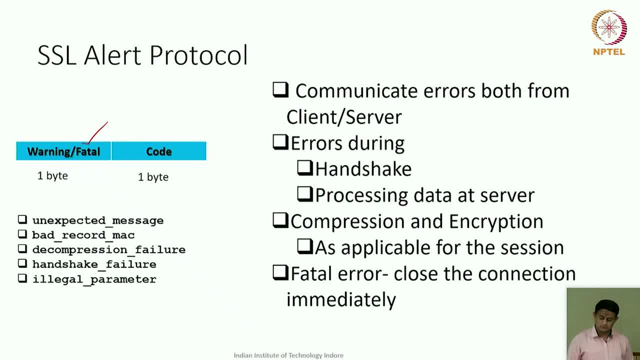 fatal. so if it is a fatal error, then the two parties need to end the communication immediately. so either it is a warrant or it's a fatal. if it is a fatal kind of error, then it's actually the connection is terminated. and the important thing is these alert protocol messages. they are: 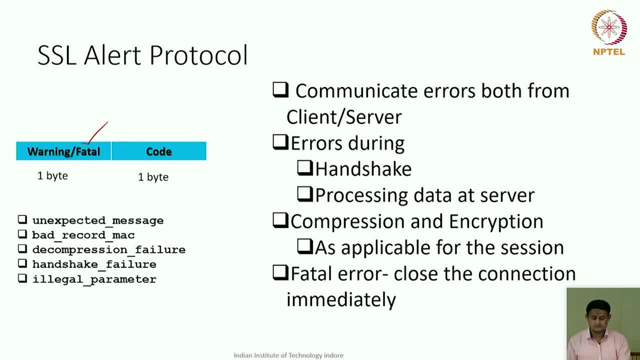 of the two bytes. the first byte indicates what kind of the error or the message it is, and the second byte it has got a code, so that code is actually taken and then interpreted. what is what you need to do with respect to the existing connection? and these messages, in fact, are also. 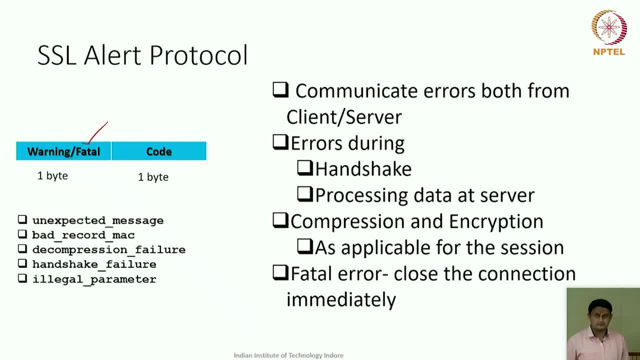 encrypted and asked as per the ongoing communication. so you establish a ssl connection between two endpoints using some kind of encryption algorithm and some algorithm for the mac calculation or hash generation. you so using the same mechanism. you also use some compression algorithm. whatever you encryption algorithm or compression algorithm that you use for encrypting the data given by the application. 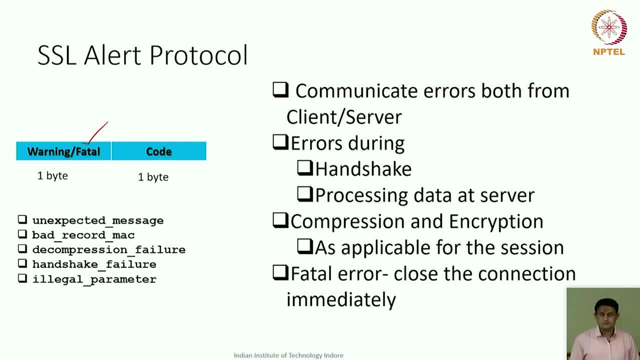 the same set of algorithms can also be used to encrypt and compress the ssl protocol message as well. so the same two bytes are taken and then I don't know how much compression it's actually used at the end, but you can in fact use that encryption compression with them. 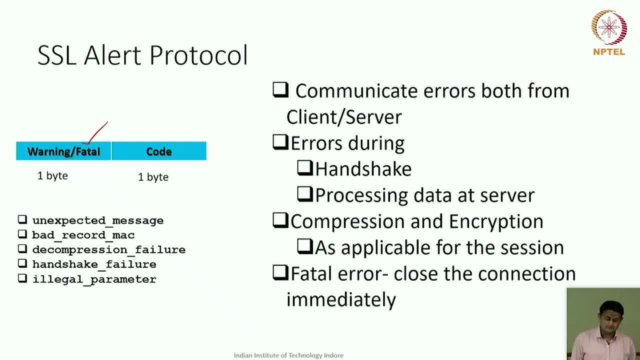 so there are a bunch of error types and the correct codes. so these are the common fatal errors that you can see. so unexpected message which is not supposed to be received. bad record mic- the mac actually calculation fails at the other end. then the other party can tell that I cannot actually understand this. can you send it? or if the 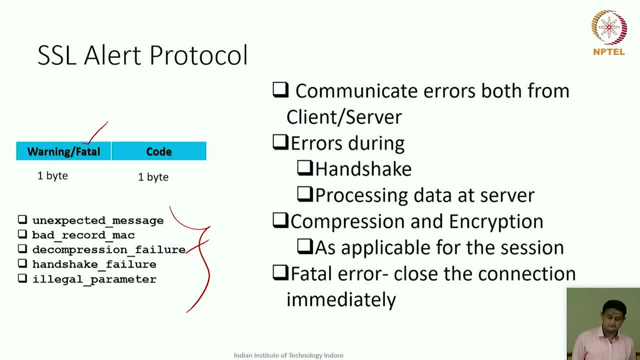 compression algorithm fails, then also it can indicate that the decompression could not be done or the handshake is used for establishing connection right at the beginning. If there is an issue with the establishment connection itself, that time also it can use. and if there are some illegal parameters that are passed to the SSL communication channel, then 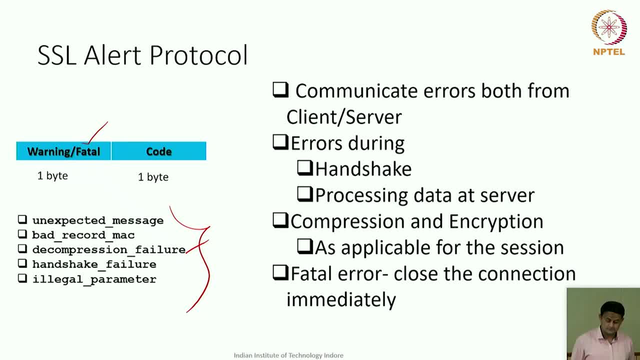 that can also identify this. We will see what kind of parameters are transferred during the connection establishment and other phases. So that is what the SSL alert protocol is all about. Very simple protocol, only two bytes: one is indicating the warnings and the second one is the code. 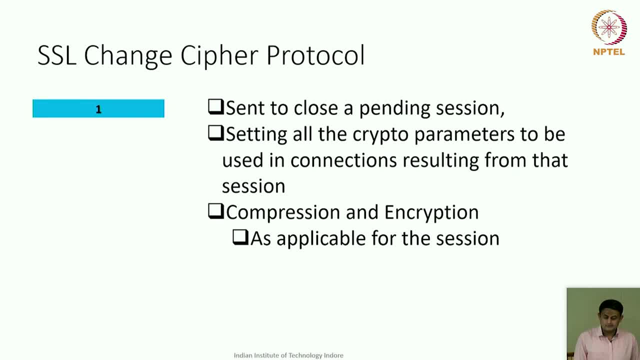 And even simpler. management protocol in the SSL suite is basically one byte data that gets transferred, called as the SSL change cipher protocol. This protocol is used when you want to terminate an existing connection. whenever the tunnel is established with two end system, you want to terminate that. that time you can send this message or during the ongoing 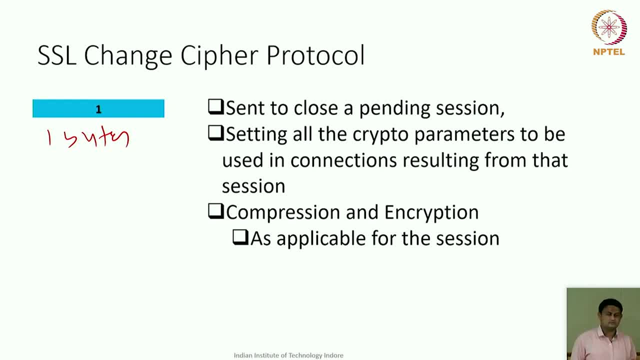 conversation. if you want to change some of the algorithms that are used. for example, the encryption algorithm need to be changed, the compression algorithm need to be changed. it is as good, as I no longer want to use this set of the protocols, but I want to switch to. 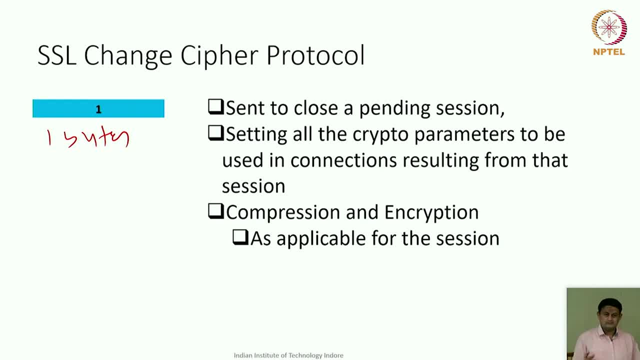 something else, So that kind of the or the key: I want to renew or change that that time also you can use that, particularly any changes in the ongoing communication you want to make, including the termination. that time you use the this protocol. And, interestingly again, although 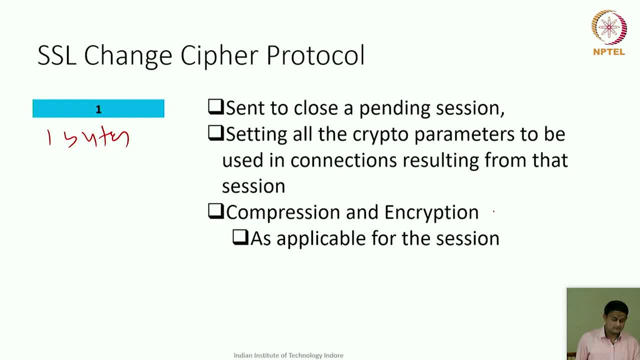 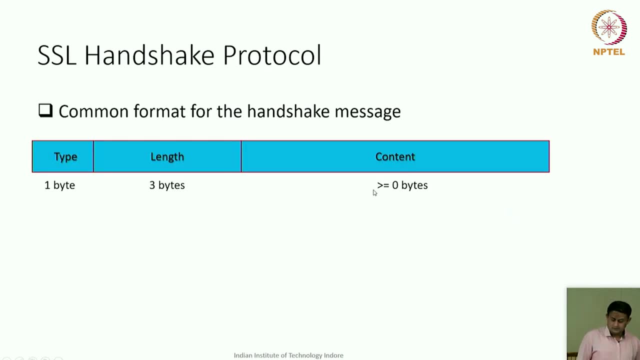 this is a one byte protocol. the same encryption and the compression method that are used for data is also applicable for this communication as well, when the data is sent to using. So the third management layer protocol, which is the most complex one out of the three, is something called SSL handshake protocol. Before we actually go in, 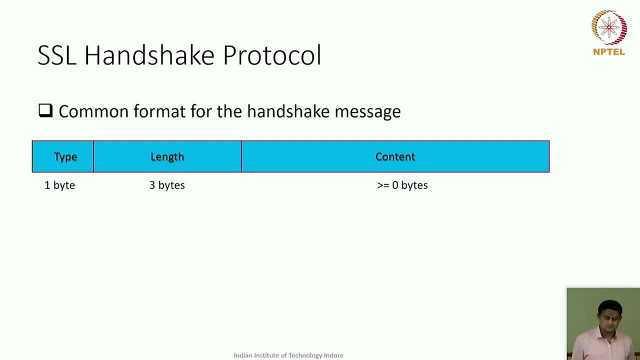 details. let us look at its structure. So this SSL handshake protocol has got three components. the first component is the type message, that is, the one byte, and then second component indicates the length of the message. whatever is carried here, so that length is indicated is here and the actual. 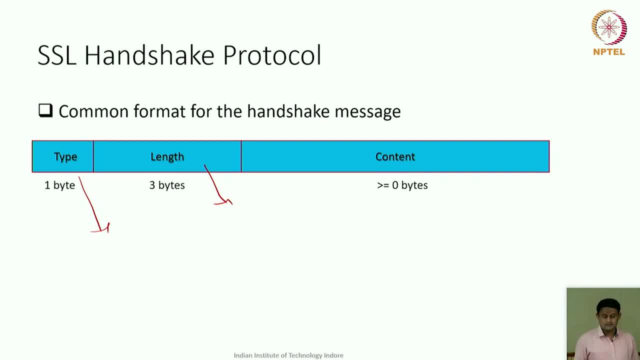 length was here. So why this type is? basically to identify whether what the client is sending to the server and the server is sending back to the client. So I just give an example. so at the time of the initial communication the client and server might exchange certificate. so it might tell this: 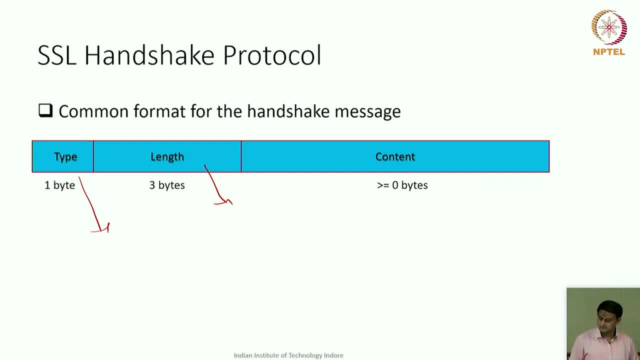 is the type of the message. they might also exchange the some random number selected to generate the session keys, So it actually identifies what kind of the message it is. So in the next slide the details are there. what all kinds of messages are there. So all of them use this generic structure. 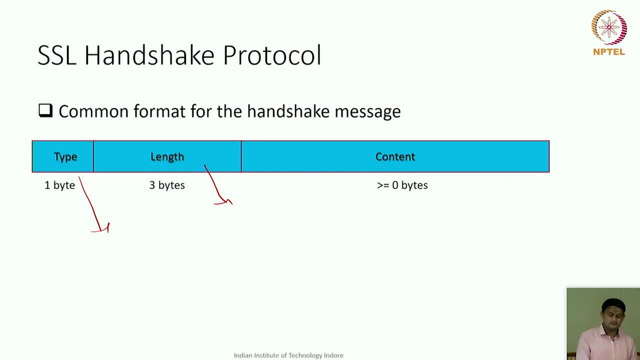 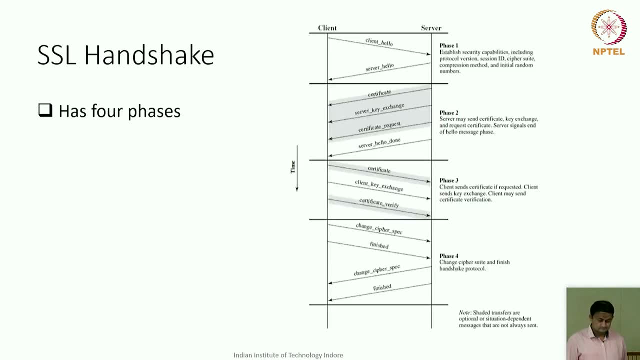 these three components. The first two are fixed: one byte and three bytes. the content itself can be of either zero or more length. So SSL handshake protocol is a management protocol. it is, as I say it is, quite complex. It operates in four pages, So phase one, phase two, three and four and these four pages. 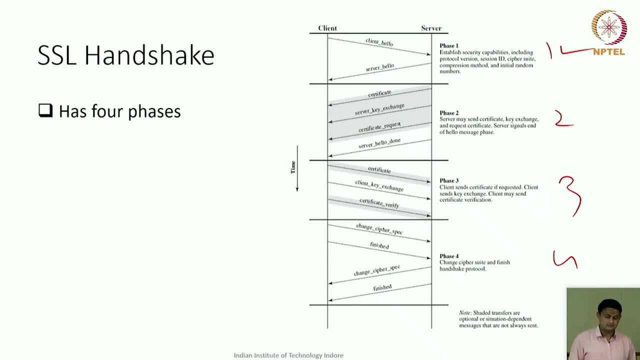 in the first phase. basically client and server. with respect to the HTTP, if you talk about, they say that hello to each other. we do want to. I am so, and so I want to talk to you, and the server says I am so, and so I am also willing to talk to you. 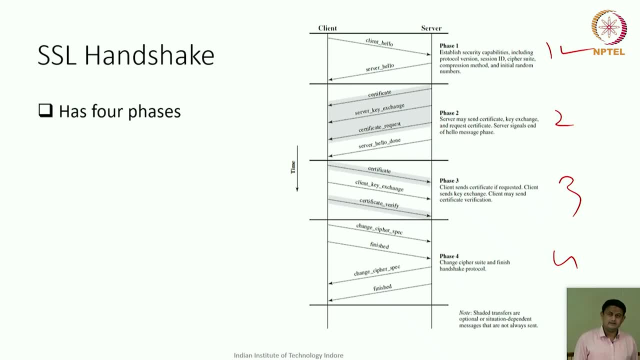 And in the second phase the server might send its own certificate to the client, basically to authenticate, to establish that the client is indeed communicating or establishing connection with a genuine server. So the server sends a bunch of details back to the client. In the third phase, sometimes the client might also send a certificate to the server. but 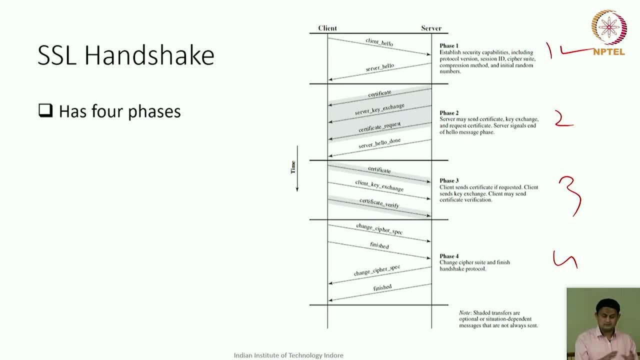 that is an optional thing, and in the process they might also derive something called session key. So that session key is used for encrypting the data. The certificate has got the public key information of the peer, but that key is not used for data encryption. 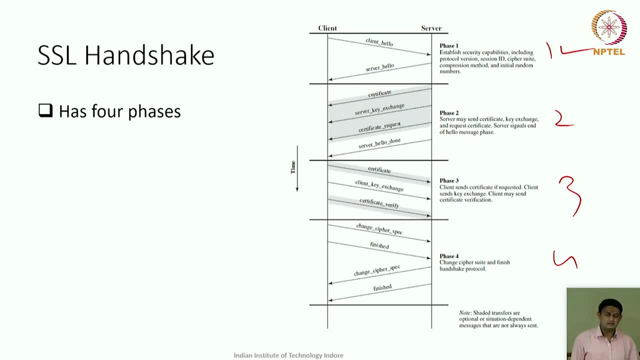 Data encryption happens using a simulation. It is a symmetric key algorithm and to that you give a session key as an input. So in the third phase that is actually calculated and derived and in the final phase you negotiate: okay, this is the key that we are going to use and this is the method algorithm we are. 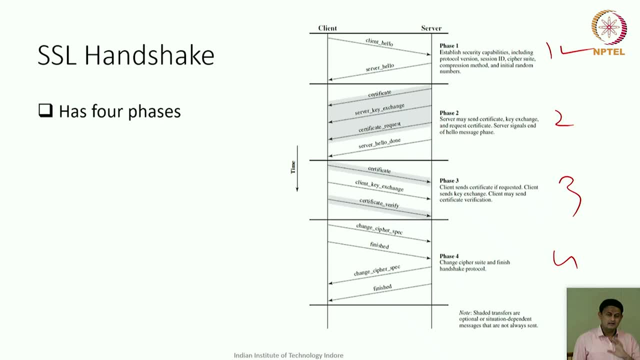 going to use for encryption, for example, DES, and then this is how we exchange the key: all the parameters- This is the compression algorithm that we use- All those crypto parameters are used. Okay, All the parameters are, and the algorithms are negotiated, and then it's done. 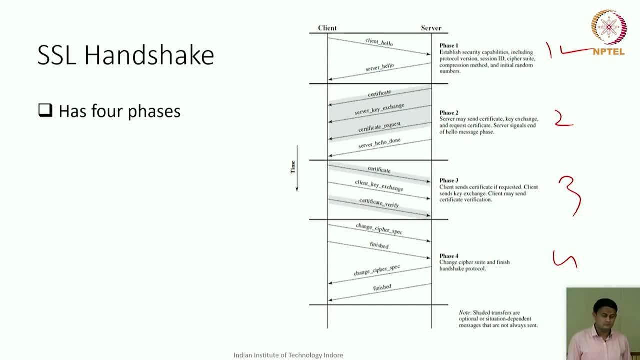 In the fourth phase they hang up, So we are all set to go now, and now we can communicate with each other. So that is roughly what happens. So let's go and look at the details of what exactly happens in each one of these four. 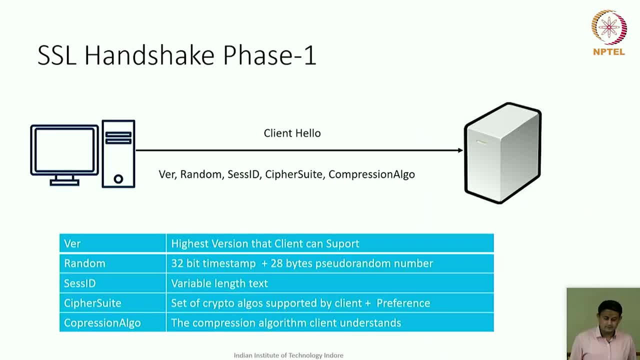 pages. Let's begin with the phase one In the phase one. phase one is initiated by the client and the message is sent to the server and that message has got these five quantities. The first message identifies the version number of the SSL protocol that the client can support. 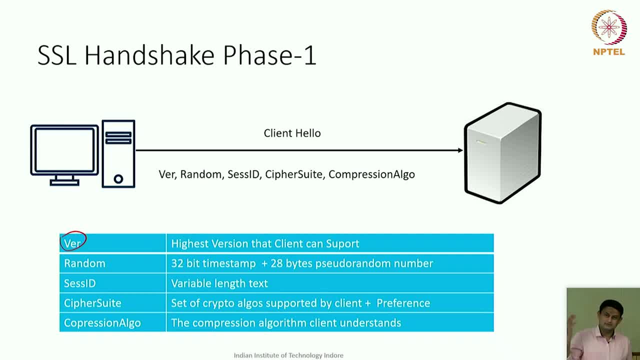 This is the highest version, meaning if the client can understand only version one and two, it will tell I can understand version number two. So, assuming the backward compatibility is there, the server can either choose to talk to the client with version number one or two, either of that. 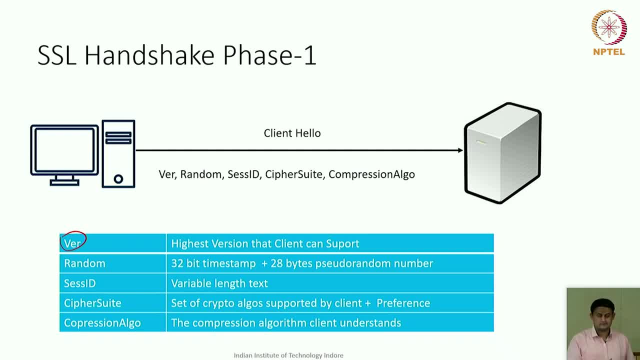 So in any case, the client, whenever it sends a message, it identifies the highest version that it can support, maybe 3.0,, 2.9, something like that, And the second quantity is something called the random number. So this random number has got two components. 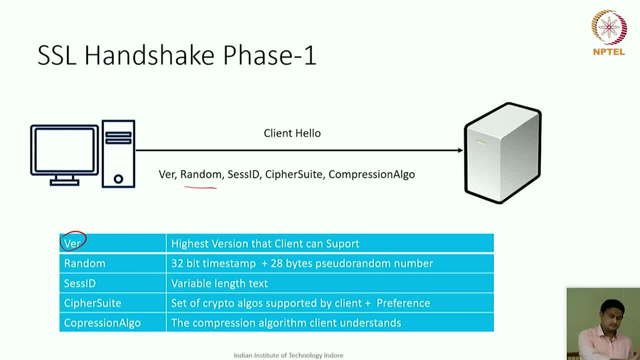 One is the 32-bit timestamp plus another 28 bytes of the pseudo random number. This is generated with the random number. You take the timestamp value from the system clock plus the 28 bytes you take from the random number generator. These two are sent as one entity to the peer, basically, in this case, the server. 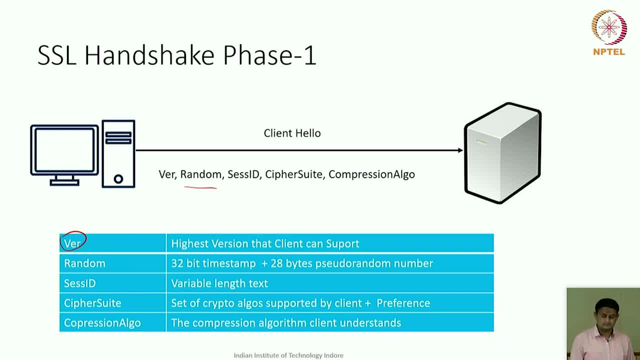 So why this is required? This is required basically to derive subsequently the session case And the session itself is identified by a session ID. This is a variable number. This is a variable number. This is a variable length. text might be having the only number and alphabets as well- a combination. 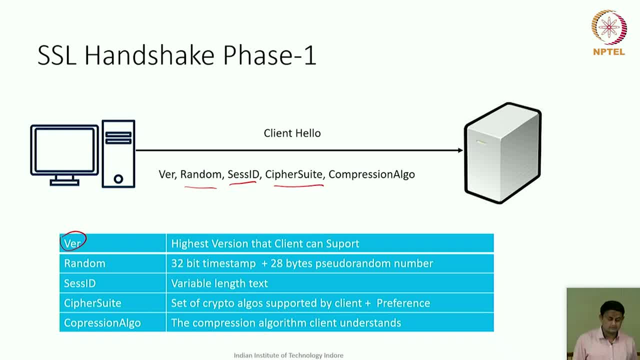 of them. And the fourth parameter is called CyberSoup. It is where the set of the cryptographic algorithms and the key exchange methods that the client can support it exports all of them to the server. So these are all the things that I am going to understand. 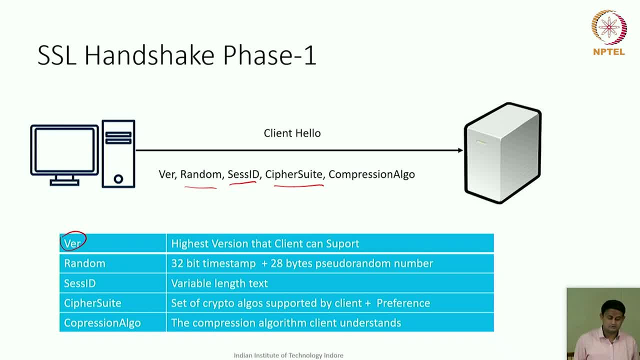 I can use these many numbers of protocol. And the last thing is the compression algorithm. Which compression algorithm? Let's say you have got a bunch of compression algorithms. I can understand compression algorithm number 1,, 2,, 3 or whatever, all of them. 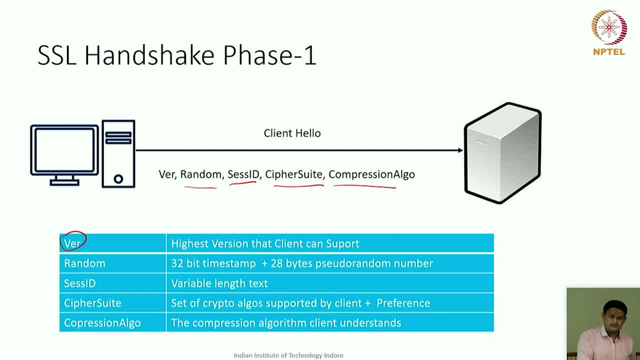 So one more thing: when it identifies the set of cryptographic protocols that it can understand, the client actually orders them in the order of their preference. So the Maybe The Crypto Algorithm 1 is the preference number 1, Crypto Algorithm 2 is the preference. 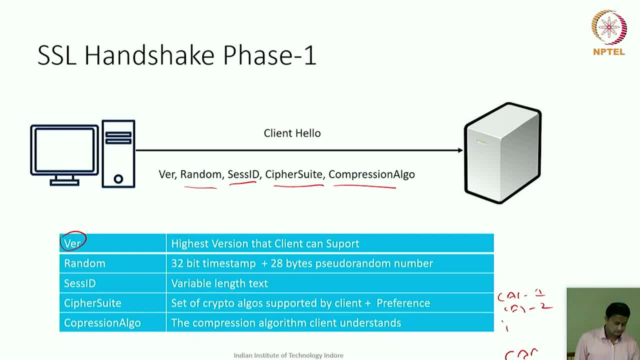 number 2 and so forth. Crypto Algorithm: number n and this is the preference number n. So why this is numbered prepared? So when the server takes it, it understands that the client wants to use this highest number, assuming 1 is the highest priority element or the algorithm. so the client wants. 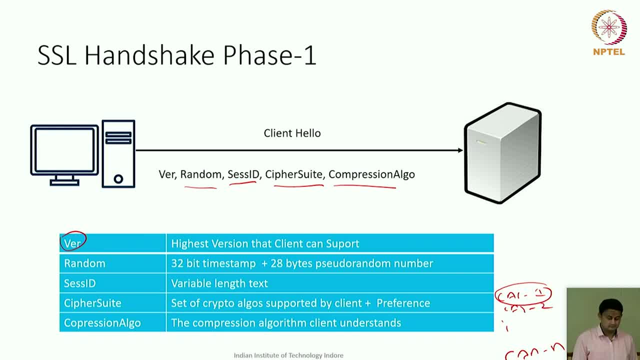 to talk with using this protocol, this algorithm, So maybe if I support that, then I can use that as well when we start engaging in the conversation. That is the meaning of that. So these five quantities are sent as part of the client hello message. 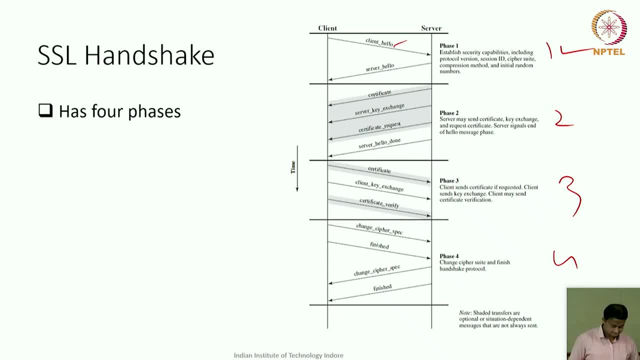 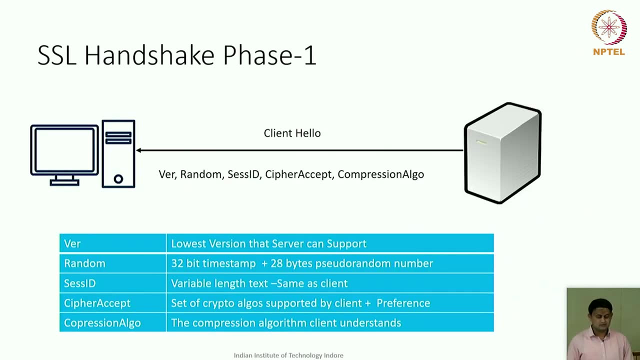 So remember, client hello message is the first, this message, And in the phase 1 itself the server also sends back a reply which is more or less the echo of what the client has sent to the server. So the same set of quantities are there. 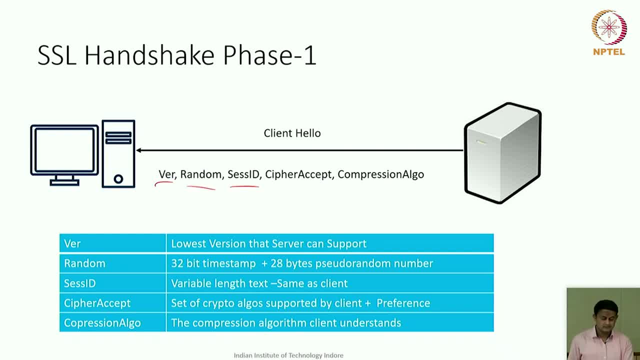 The version number is there and the random number session ID cipher accept and compression algorithm Version number is now. in the previous case it was the highest version that the client can support Here in the when the server sends to the other end. this is the lowest version that. 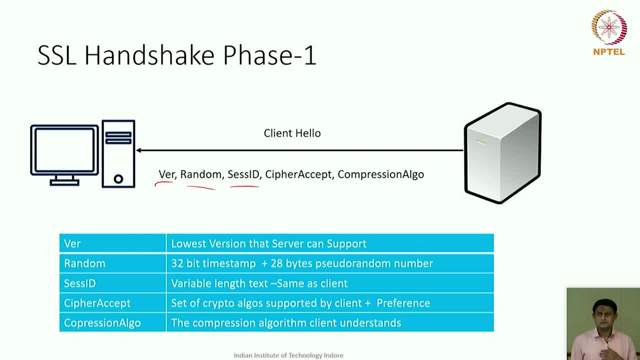 the server can support and chosen. So If the client says I can talk with you using version number 2.9, but I can also support 2.9.. If the server can also support anything below that, it actually is. whatever is the lowest. 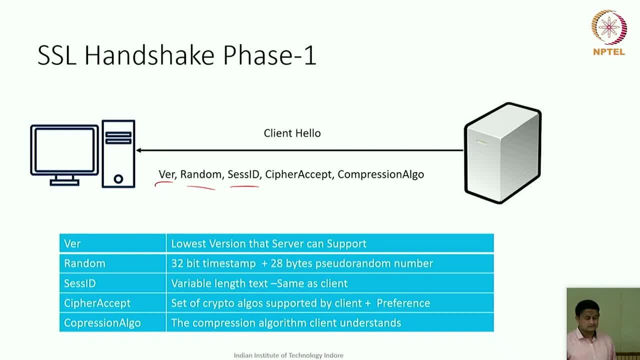 that it has got in hierarchy. it actually chooses that, and then it indicates that to the client, And then a random number which is similar to what is chosen by the client is also included here, And session ID is just echoed back. whatever the client has sent it, you just pull out. 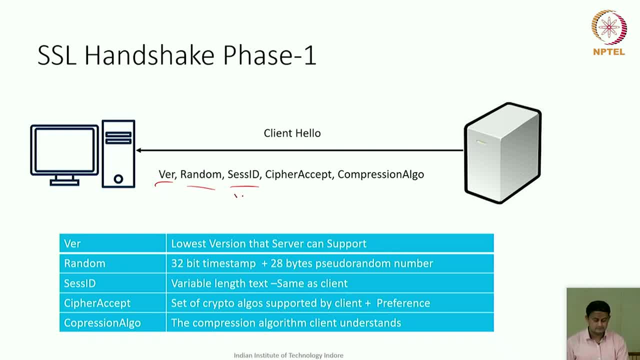 that session ID- maybe session ID in the previous case- is 10.. So this number is also set to 10 and sent it back to the client And then out of the cryptographic algorithms and the key exchange method the client has identified, the server chooses one and then usually taking into consider the preference. 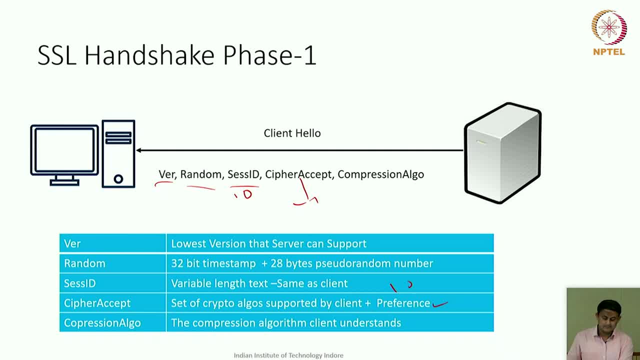 that the client has given. And then It identifies: let us talk using these protocols, these cryptographic algorithms, sorry. And then it also chooses a compression algorithm that also the server indicates in the message. So that is about the server. hello, There is a typo. this is not client hello. 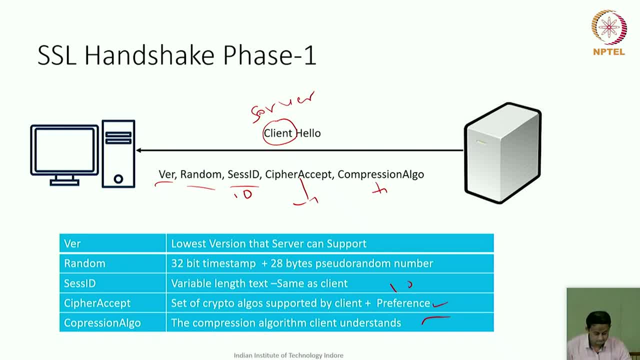 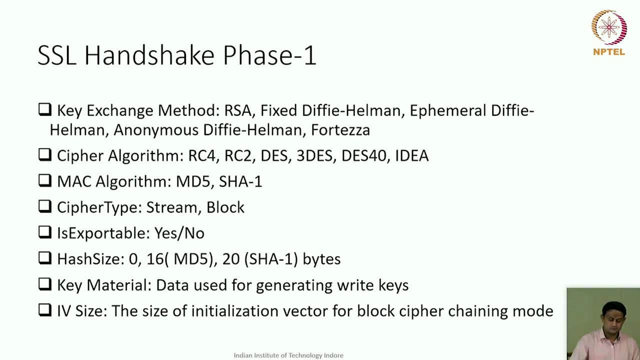 This is the server. hello. Please make a note. Yes, Thank you, Thank you, Thank you. That should take client and the server. hello. So the cryptographic algorithm, whatever the method that cryptoshoot that I was talking. So these are some of the algorithms for different purpose that are supported for key exchange. 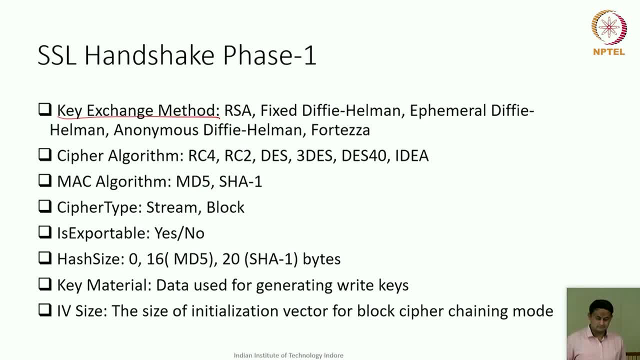 method. Key exchange method means for session key exchange methods. you can actually use RSA DP element or epimeral DP element, anonymous DP element. These are different versions that the client has selected. Okay, So these are the different versions that the SSL supports. 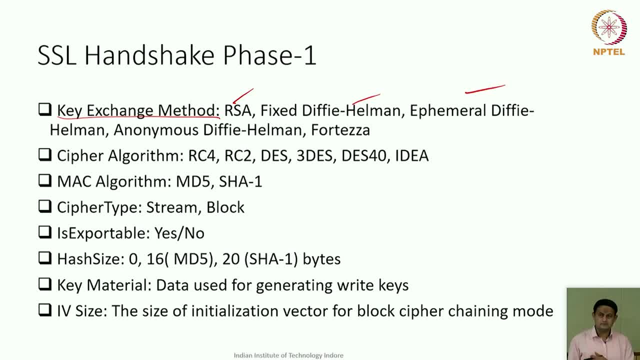 You can identify when the client sends or the server sends. we can negotiate on this one. And then the cryptographic algorithm. the cipher algorithm can be RC4, RC2, DES. These are all the supported versions in SSL, version number 3.. 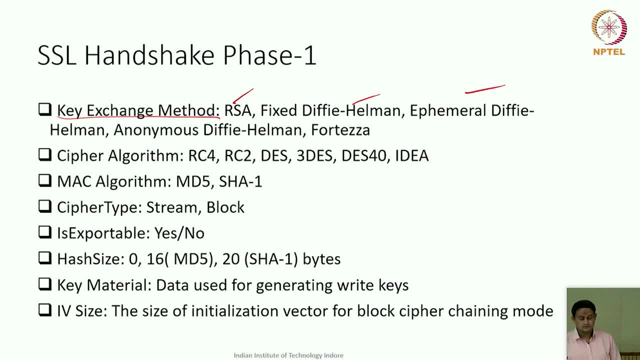 Going forward. there are few more additions that are done. And then the MAC algorithm- MD5, SA1,. you can either use the stream and then you can also use the SPAR. Okay, So you can either use the stream and or the block ciphers. 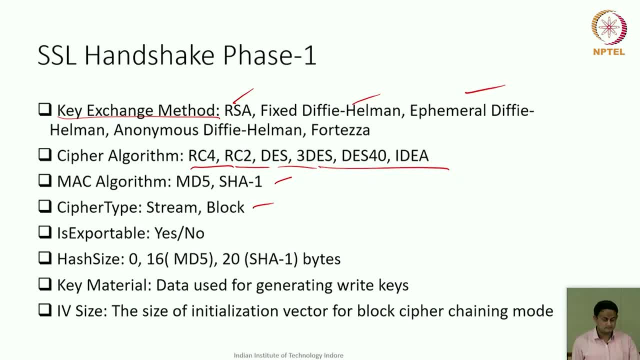 The difference between block and stream cipher is the following: If you use a block cipher- if, let's say, the algorithm takes the crypto algorithm takes some input- that algorithm is taking the fixed size input, let's say 10 bytes- And then it has got a key and it turns this 10 bytes into some output, let's say whatever. 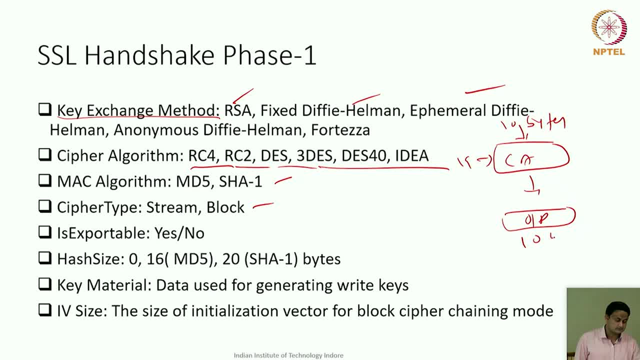 might be the length, Maybe for the sake of simplicity. Okay, Let's assume this is also 10 bytes. So you give the 10 bytes data and 10 bytes of the encrypted data comes. So if I let's say, I have the 100 bytes of the total data given by the application all. 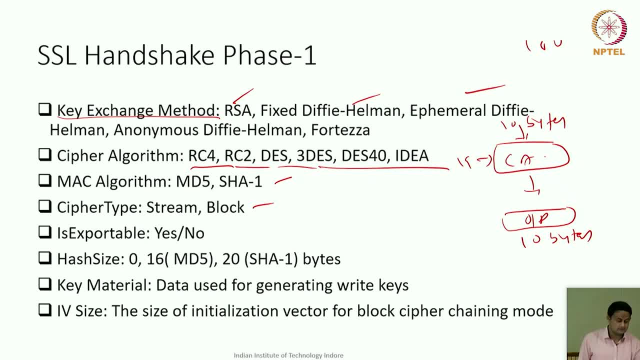 that I do is take 10 bytes at a time, give it to the cryptographic algorithm and then generate 10 bytes And second 10 bytes that other than what is used here as again given to the algorithm, in the same encryption happens, and then you get back the another. so another 10 bytes. 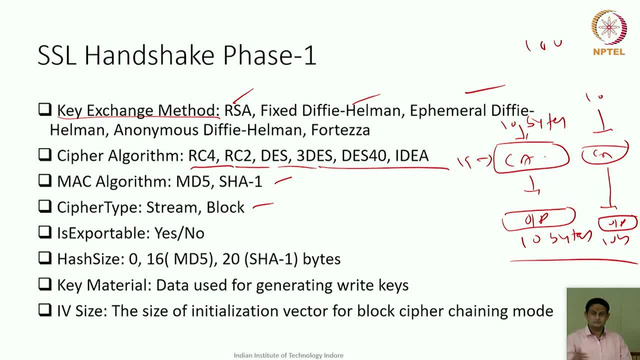 You concatenate these, all of these, and then you get one encrypted output, that is the block cipher. Every 10 bytes from the input is taken and then pass it on to the encryption algorithm. Then, whatever the encrypted data is yet, you concatenate that and then use it for transmission. 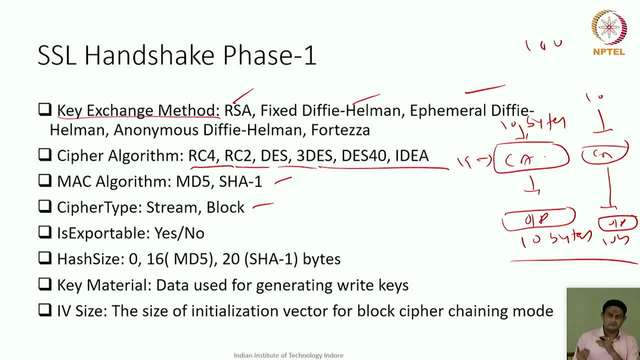 block cipher. So there is no connection between the first 10 bytes. Okay, Unlike that, stream ciphers are actually used where you got the. once you do the operation on the first 10 bytes, whatever is the output that is generated, that is also fed as input. 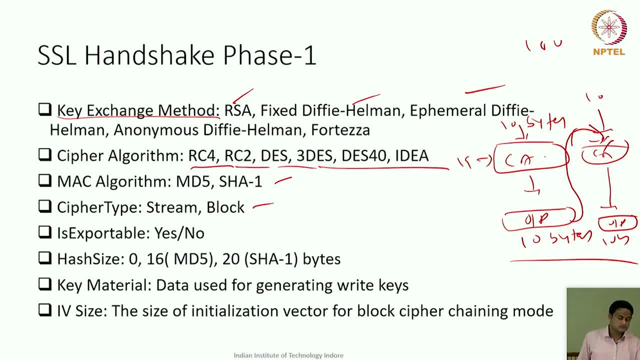 to the second subsequent operations. So that is the. so you got a chain. One is you take one thing, encrypt it and then carry that forward, Okay, And then carry that forward to the next phase and the next phase, and next phase, so forth.